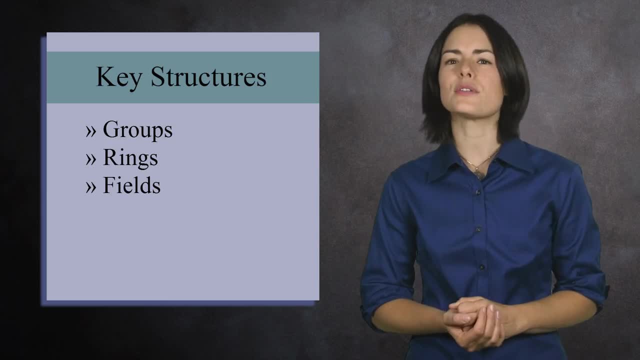 The key structures in abstract algebra are groups, rings, fields, vector spaces, and modules. You start with groups because the other four structures are built upon them. 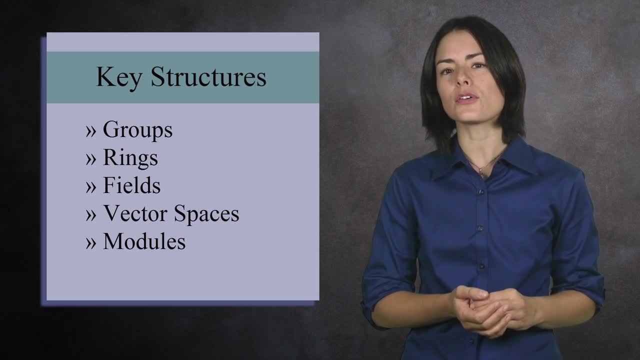 All of these concepts are fairly abstract, so it's helpful to learn lots of concrete examples to help keep you grounded and test out everything that you learn. 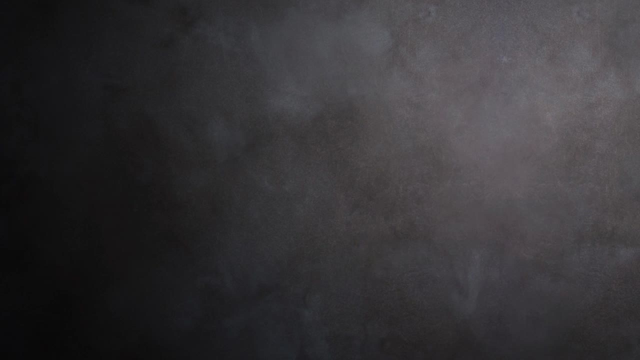 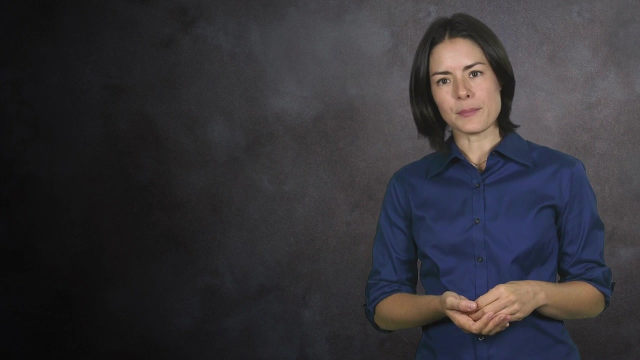 Today, let's look at examples of rings. ADDITION Before we dive into the examples, let's remind ourselves of the definition of a ring. 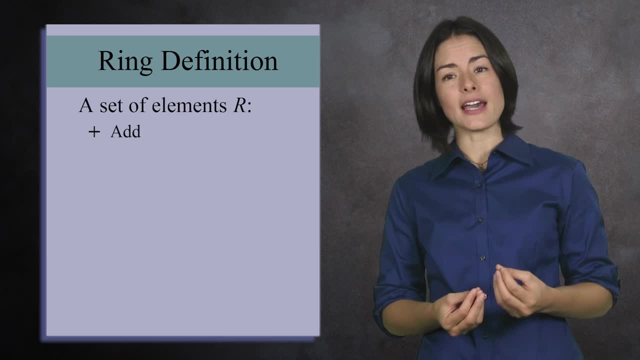 Loosely speaking, a ring is a set of elements where you can freely add, subtract, and multiply with the usual rules of arithmetic. 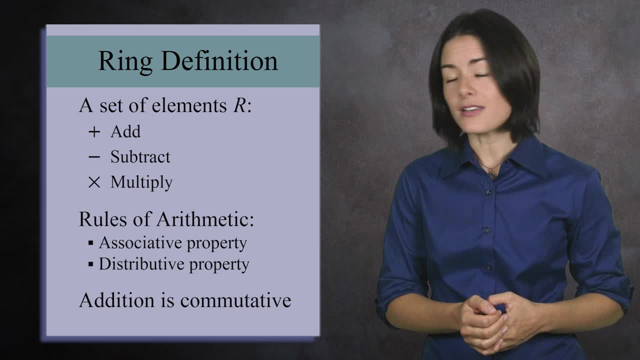 And while addition is commutative, multiplication may not be. 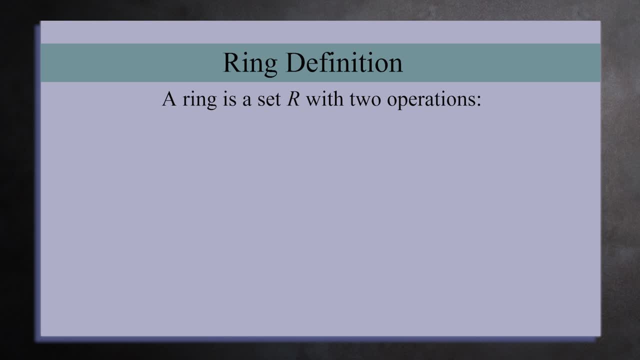 Technically speaking, a ring R is a set of elements with two operations, R is a set ofnenting numbers within留 and W is a set of elements in fortsidan. And while addition is commutative, multiplication may not be. Technically speaking, a ring R is a set of elements with two operations. addition and multiplication. 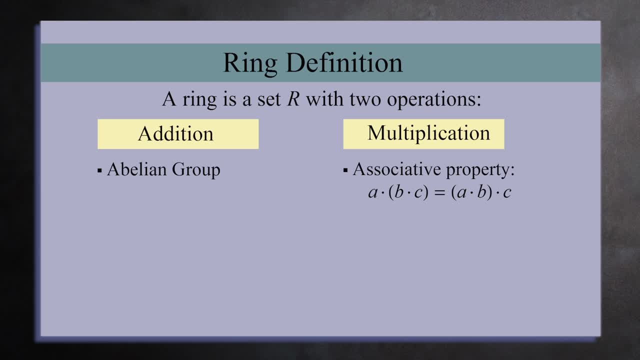 It's an abelian group under addition. Multiplication obeys the associative property. 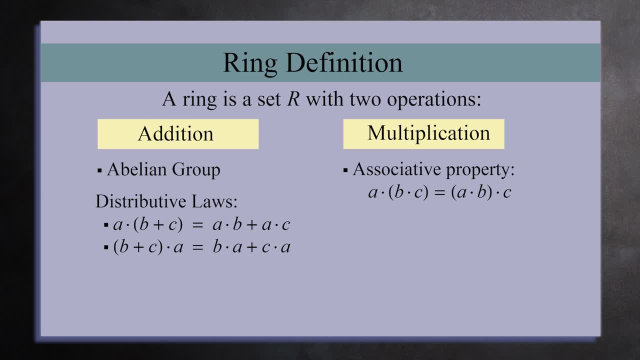 And addition and multiplication are connected by the left and right distributive laws. In a ring, multiplication may not be commutative. If it is, we call R a commutative ring. And if the ring has a multiplicative identity 1, we call it a ring with identity. Every ring has the additive identity 0, since it's a group under addition. So when you say ring with identity, everyone knows that you mean ring with multiplicative identity. 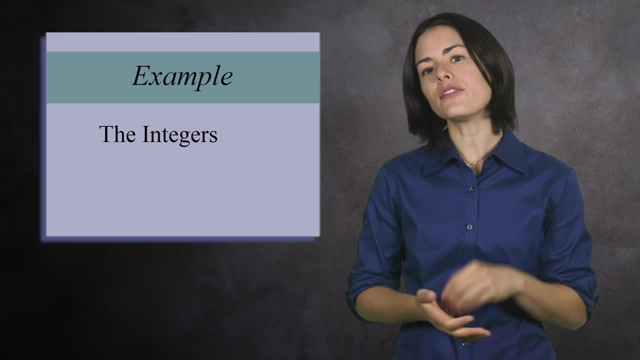 A classic example of a ring are the integers. The set of integers is denoted with a double-stroke z. This is from the German word Zahlen, meaning number. Historically, number meant integer. That's why number theory is a study of the integers. 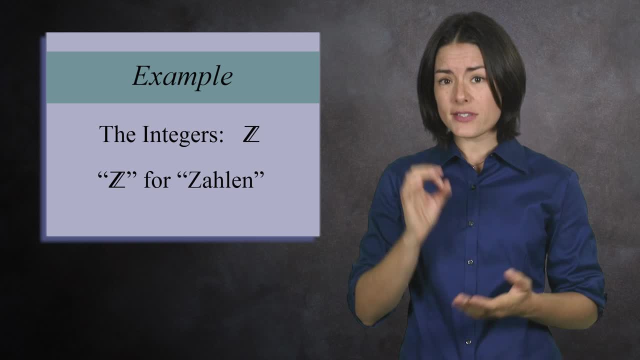 Nowadays, however, number has a more general meaning, but we stick with the letter z for the integers. Another example of a ring is a set of integers. 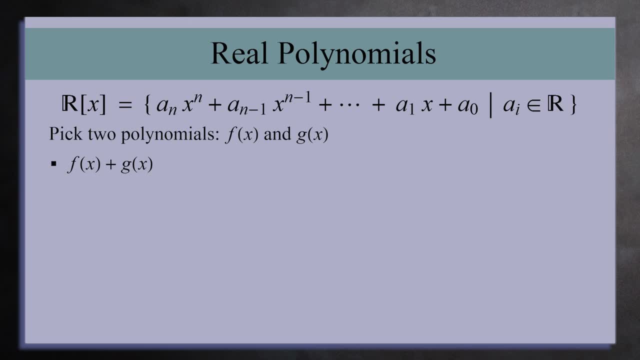 This is a set of polynomials with real coefficients. You can freely add, subtract, and multiply any two polynomials, and you'll get a third polynomial. 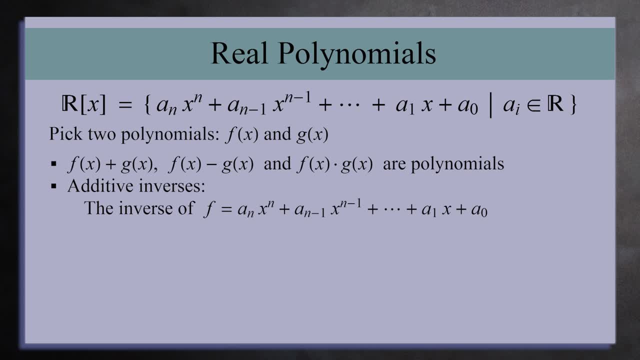 Each polynomial has an additive inverse. For any polynomial f, its additive inverse is a polynomial where you take the opposite of each term. 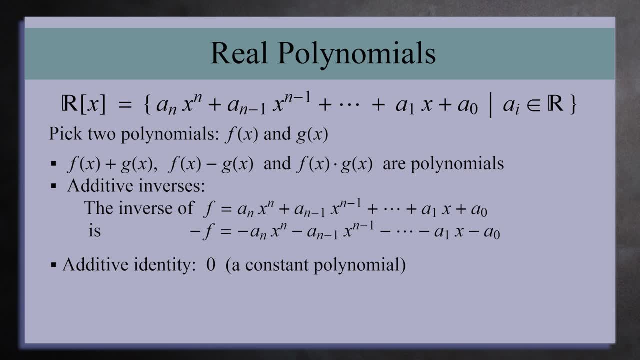 The additive identity is 0. Don't forget that 0 is a polynomial. 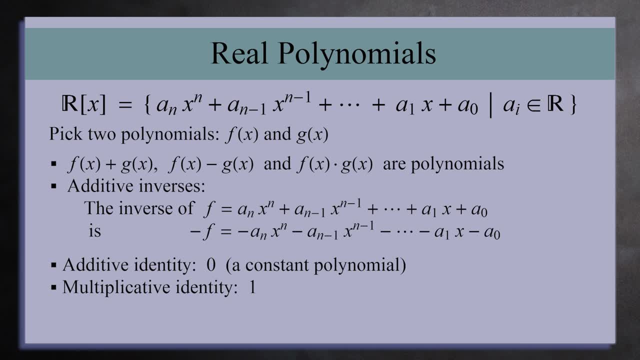 On the multiplication side, there is an identity element, the number 1, and for real polynomials, multiplication is commutative. This is a commutative ring with an identity element. 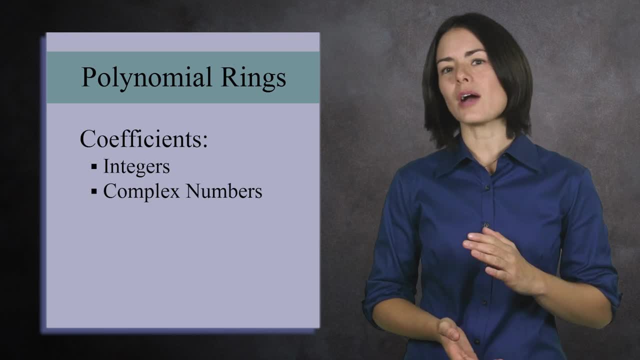 In this last example we looked at polynomials with real number coefficients. 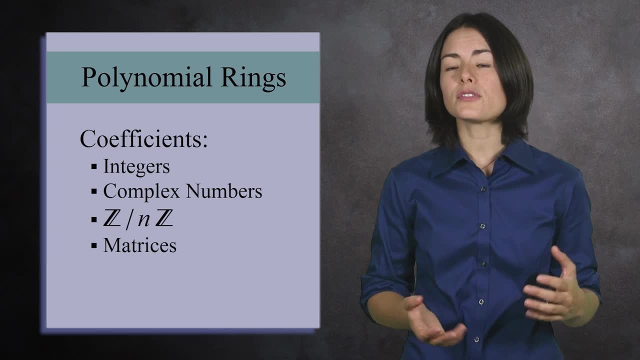 But you can use any ring for the coefficients. The integers, the complex numbers, or how about the integers mod n? 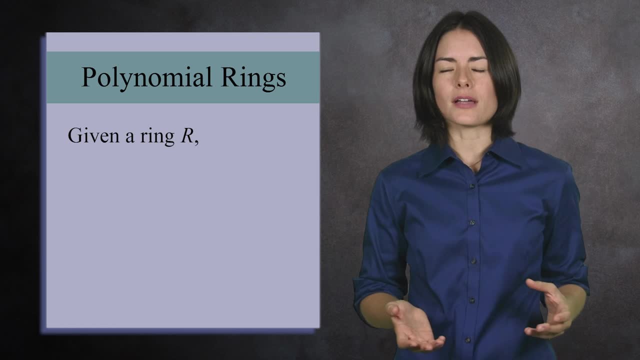 You can even have polynomials where the coefficients are matrices. Any ring will do. 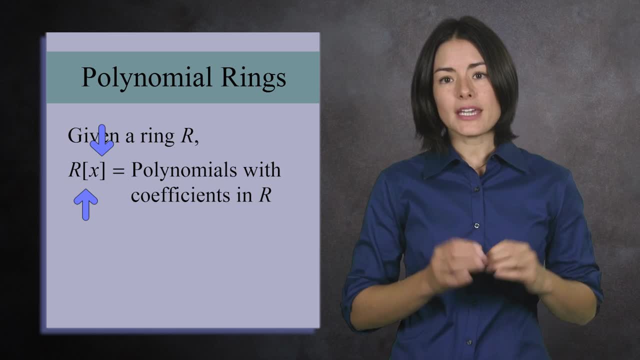 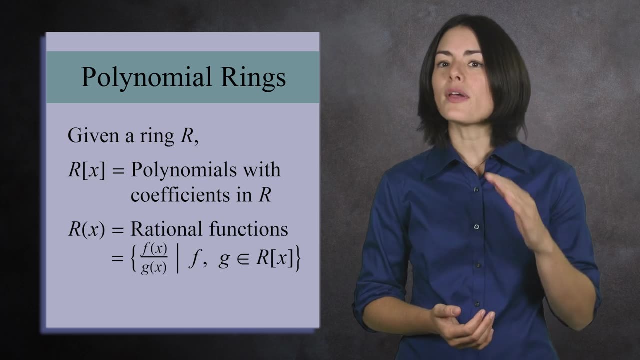 So if you are handed a ring r, you can use it to make a new ring. Be careful you use brackets and not parentheses, they mean different things. Brackets means the set of polynomials, while parentheses means the set of rational functions, 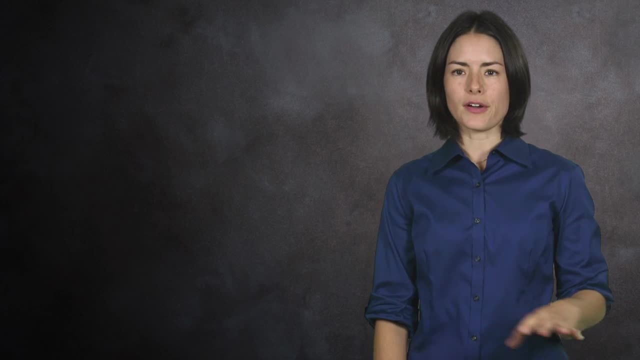 which are fractions of polynomials. So far, every ring that we've seen has been commutative, and has had an identity element for multiplication. 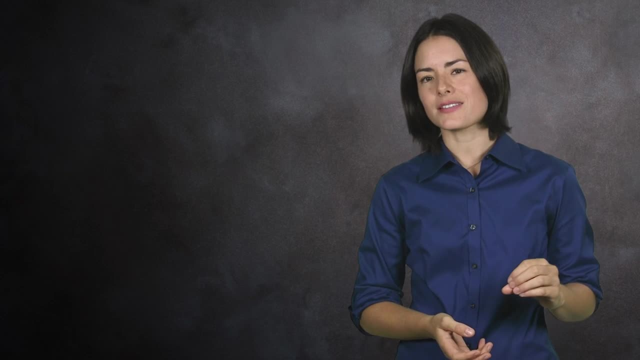 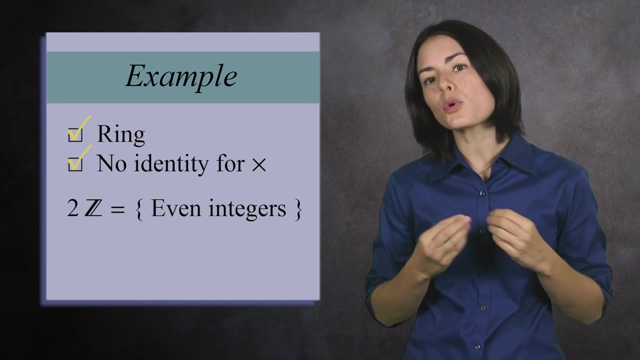 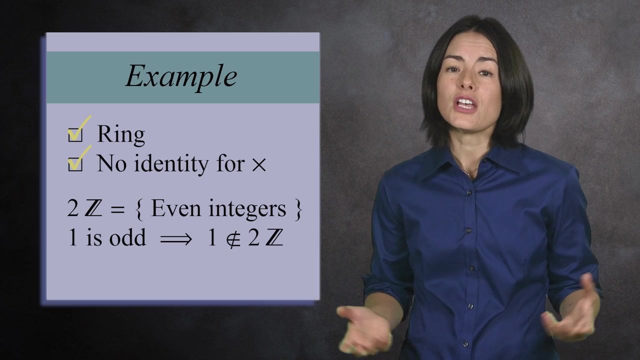 Let's now look at rings where this is not the case. An example of a ring WITHOUT an identity element is a set of even integers. If you add, subtract, or multiply any two even numbers, you'll get another even number. But the number 1 is not in this set because 1 is odd. 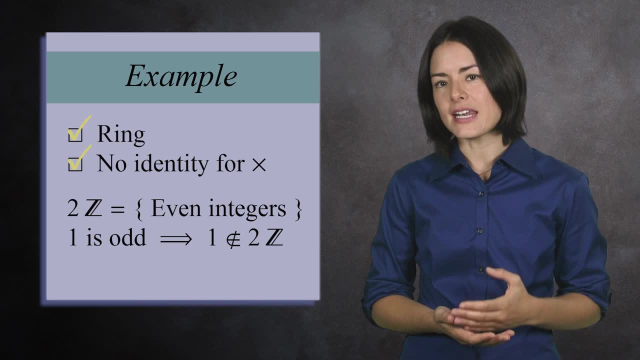 So while this is a commutative ring, it does NOT have an identity element for multiplication. 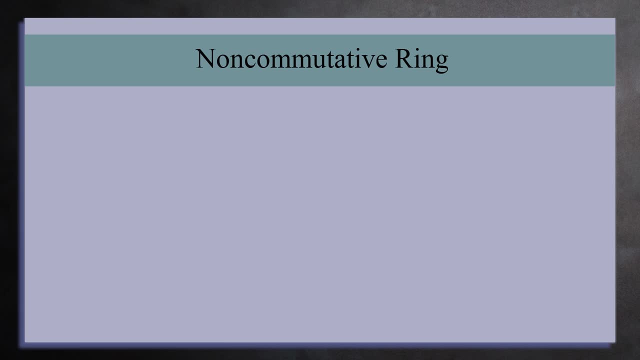 Let's now look at a ring that's NOT commutative. The classic example here are matrices. For instance, the set of 2x2 matrices with whole number entries are a ring, but it's NOT commutative. 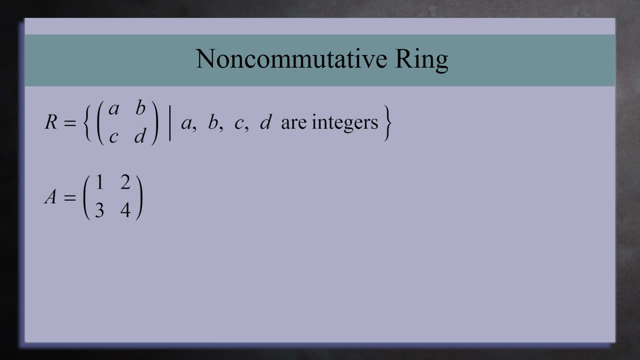 To see why, consider the two matrices. 1, 2, 3, 4, and 1, 0, negative 1, 1. Here, a times b does NOT equal b times a, so this ring is NOT commutative. 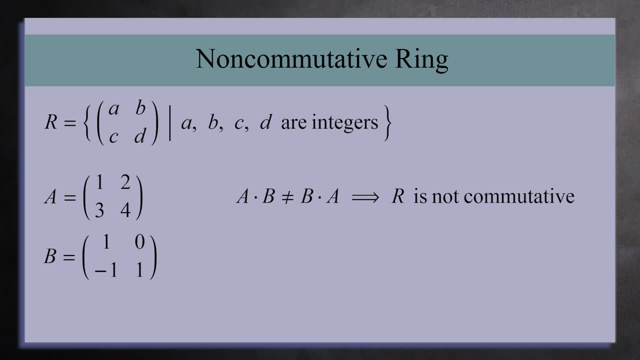 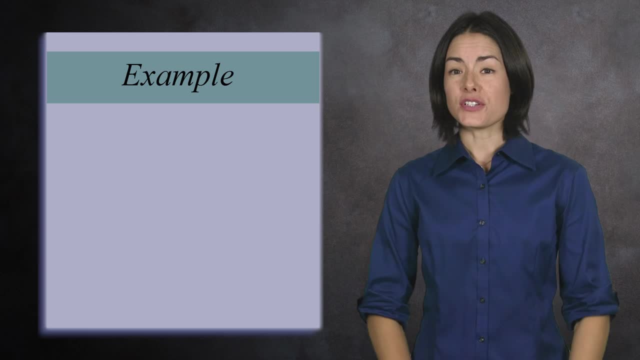 We call this a non-commutative ring. As a consolation prize, however, it DOES have an identity element. The 2x2 identity matrix. 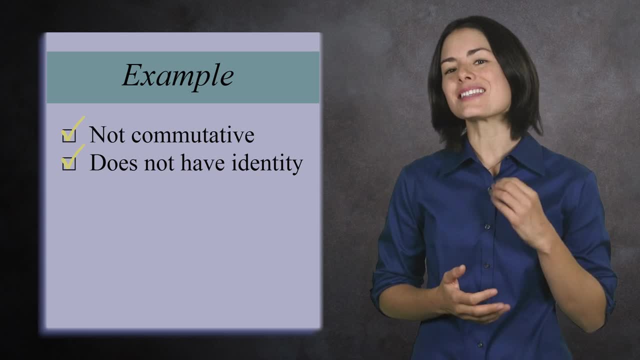 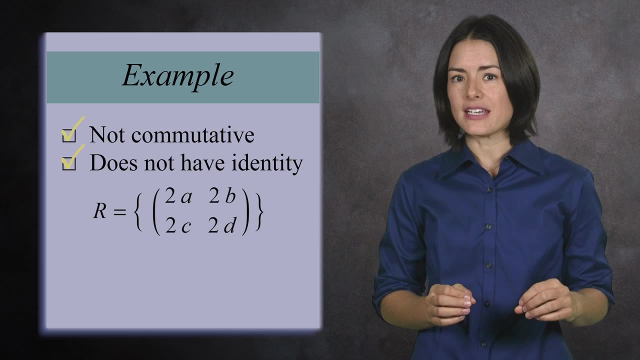 Just for fun, let's see a ring that is NOT commutative, and does NOT have an identity. The 2x2 matrices with even entries. This definitely does NOT have an identity, since the identity matrix has 1s along the diagonal, and 1 is an odd number. 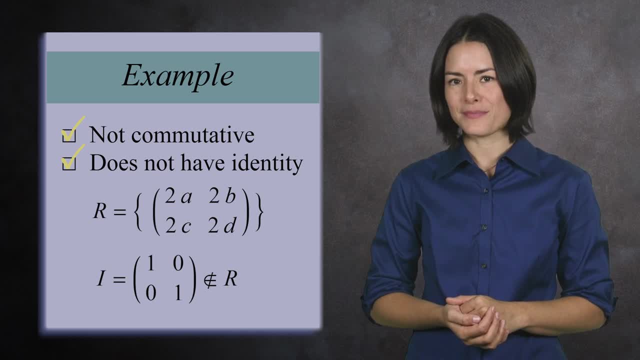 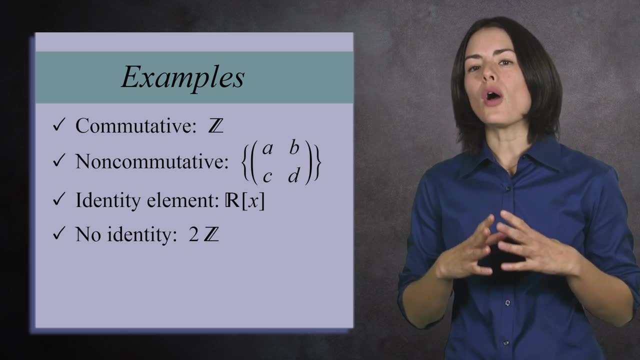 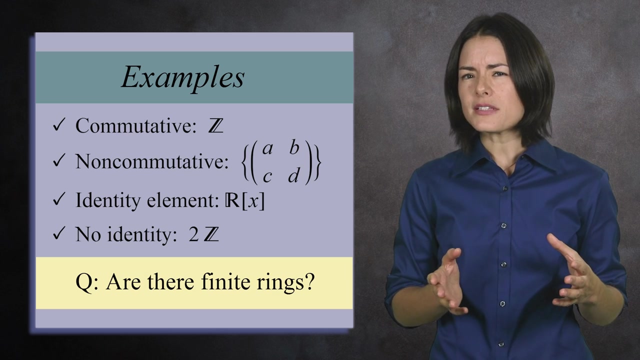 This poor ring is having an identity crisis. Already we've seen a wide variety of rings. Commutative, non-commutative, identity, no identity. But all the examples have had something in common. They have all been infinite. Are there rings with only a finite number of elements? I'm glad you asked. Because yes, yes there are. 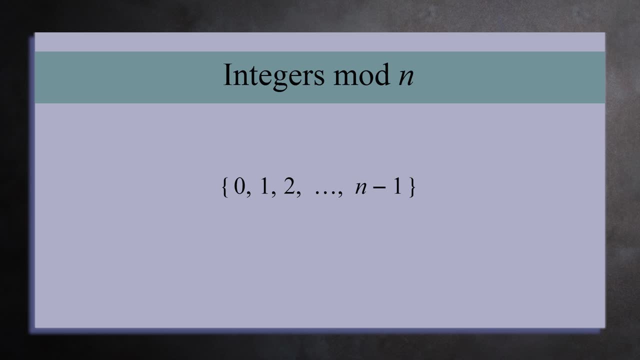 The integers mod n are a finite ring with only n elements. 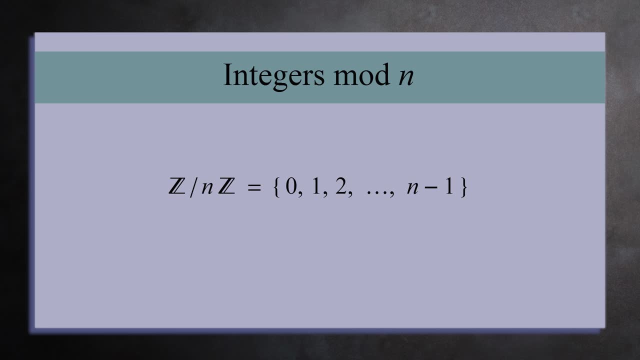 Here is the notation for this ring. You may recognize this from your study of groups. This is the notation for a quotient group. Z is the group, and nz is a normal subgroup. The quotient group is the group of cosets. This notation is carried over to rings. Here, z is the ring, and nz is an ideal. In this context, we call it a quotient ring. The integers mod n is a finite ring. 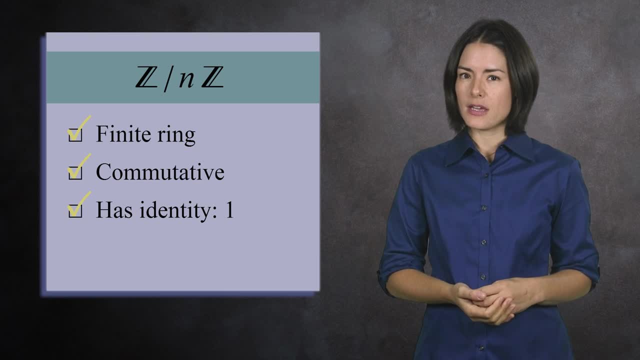 It is also commutative, and contains an identity element 1. This gives us a nice list of finite rings. The integers mod 2, mod 3, mod 4, mod 5, and so on. 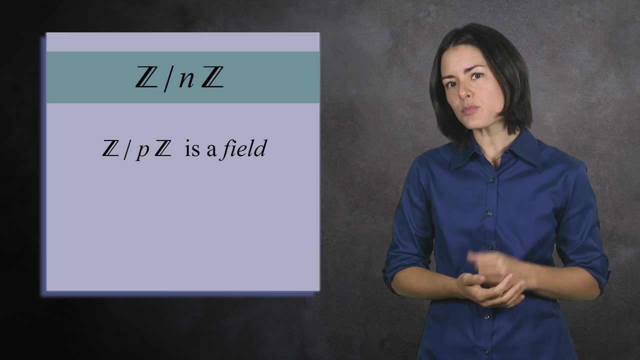 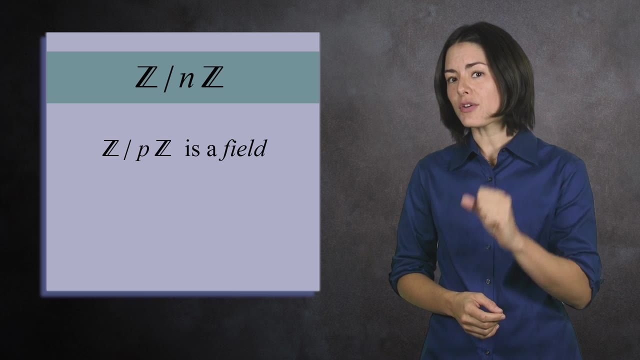 But something special happens when n is a prime number. If n is prime, the integers mod n is now a field. Here's where you need to be careful. Every field is a ring. But not every ring is a field. 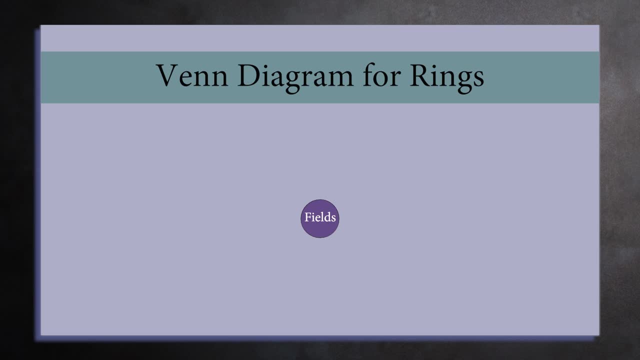 If you were to draw a Venn diagram, the set of all fields would lie inside. 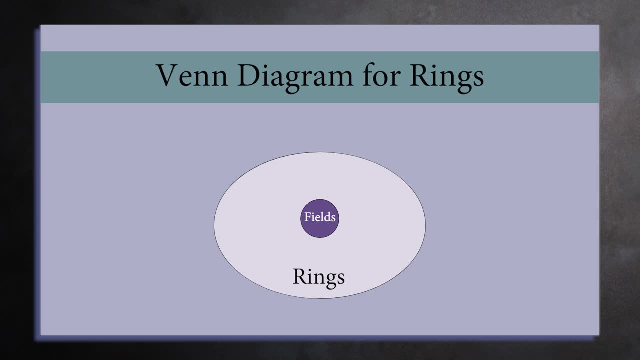 The set of all rings. And since every ring is a commutative group under addition, the set of rings lies inside the set of groups. 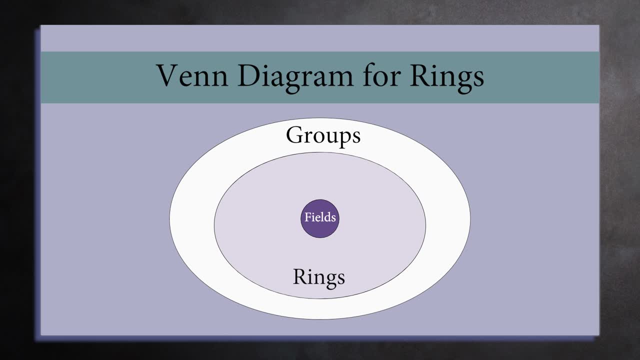 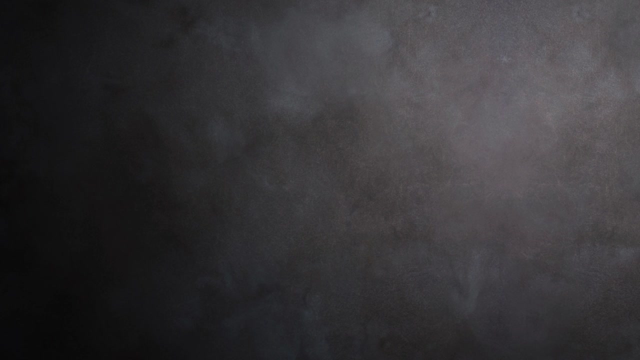 From the examples that we've seen, we can add more details to this diagram. Inside the set of rings are the commutative rings and the rings with identity. Every field is commutative and has an identity. So the set of fields lies in the overlap between commutative rings and rings with identity. 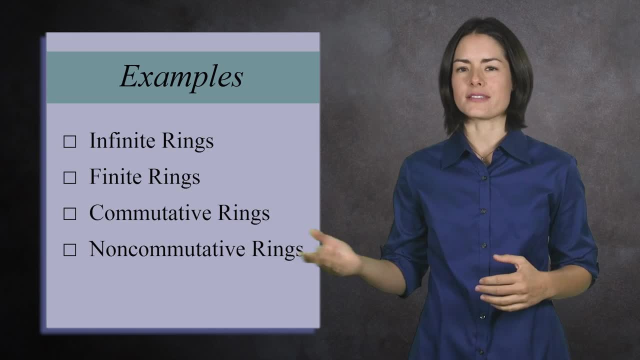 I know what you're thinking. You've shown me lots of examples of rings. 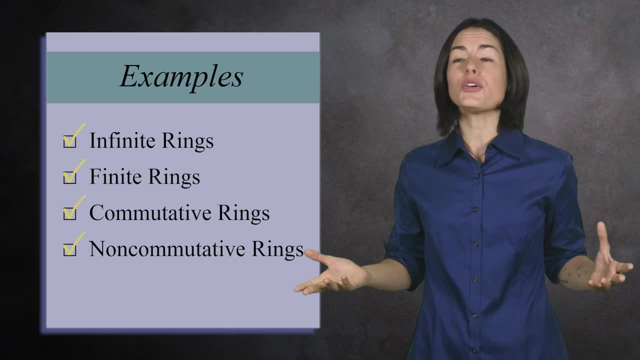 Infinite rings, finite rings, commutative rings, non-commutative rings. 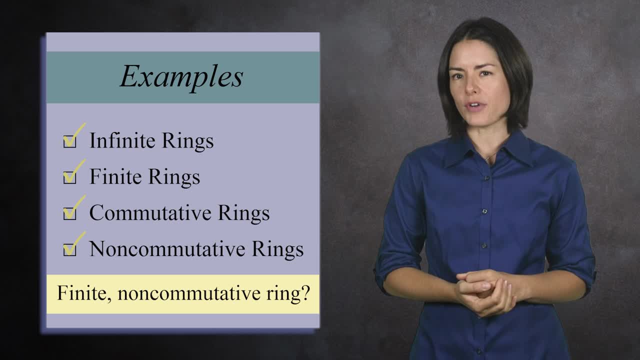 But you haven't yet shown me a finite, non-commutative ring. This I'm going to leave as a challenge for you. Here's a hint.